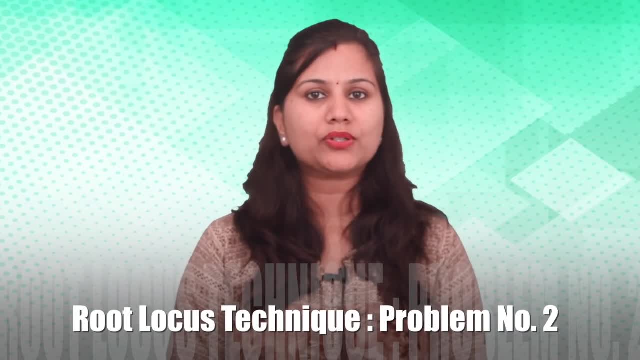 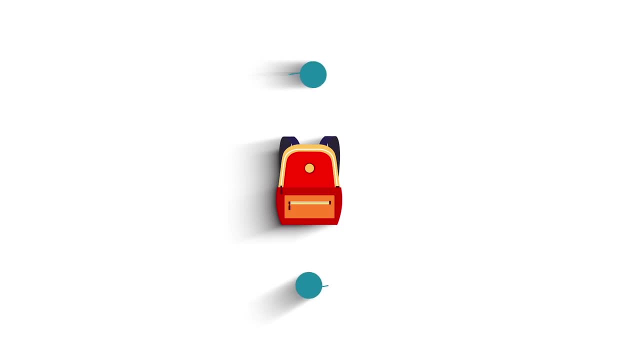 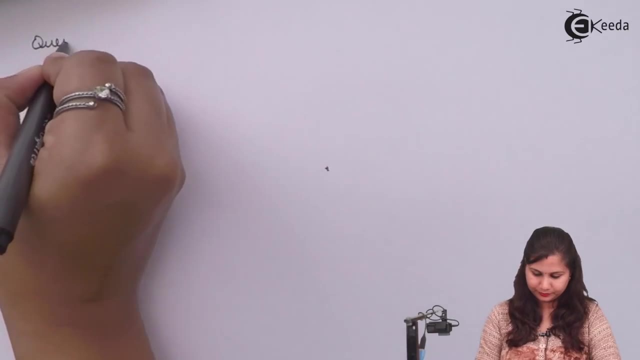 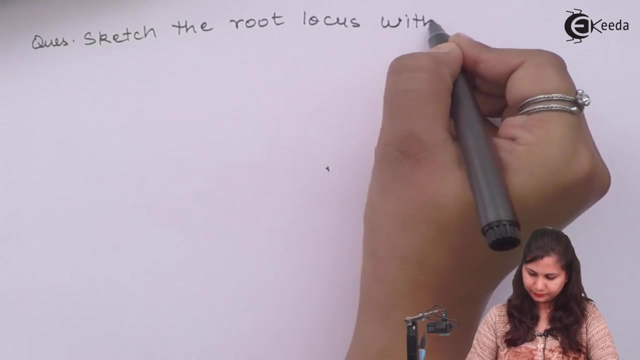 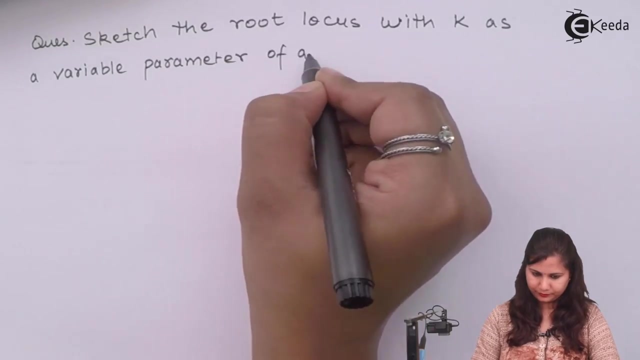 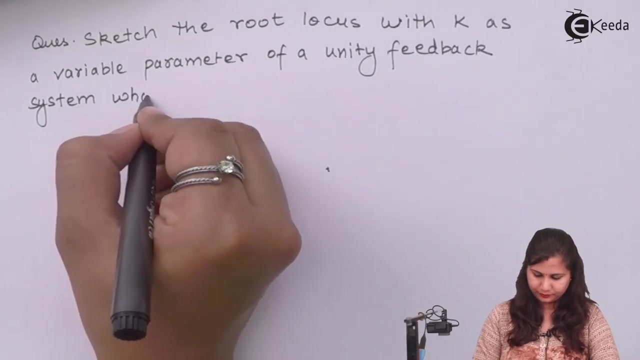 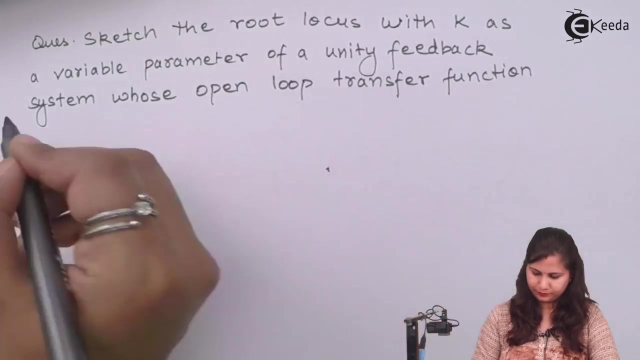 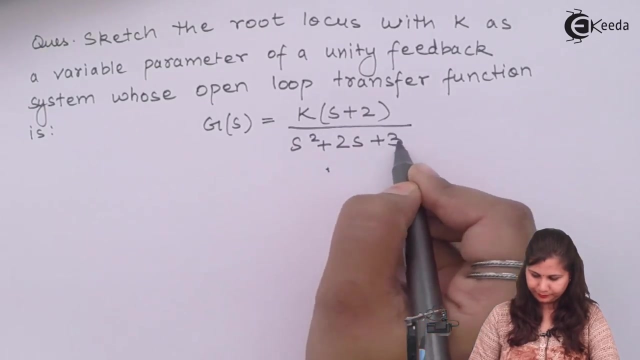 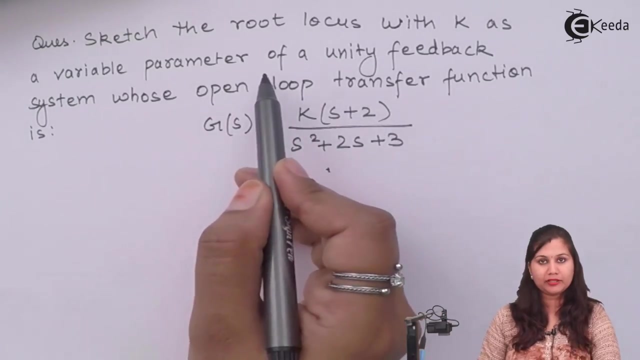 Hello friends, in this video we are going to solve a problem on root locus technique. So let's take a problem. So our problem is: we have to sketch the root locus with k as a variable parameter of root locus. So we have to draw the root locus of a unity feedback system whose open loop transfer function. 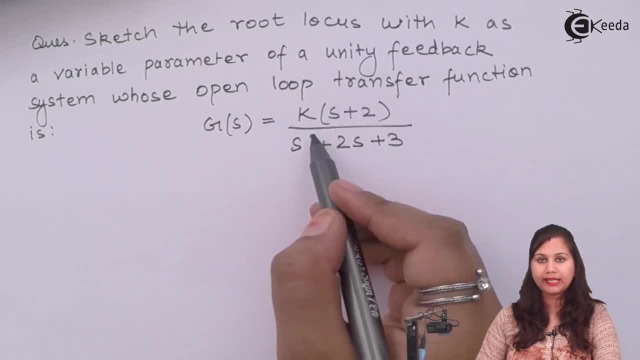 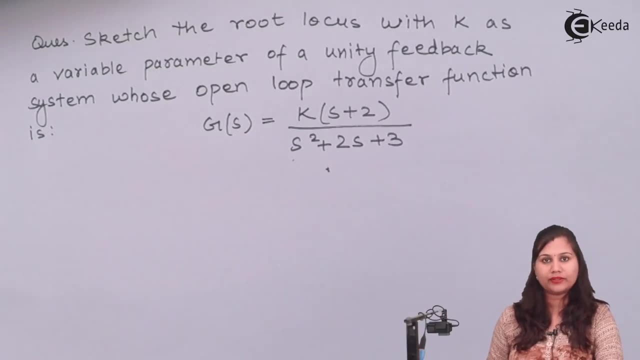 is given to us as gs equals to k s plus 2 upon s square plus 2s plus 3.. So let's try to solve this problem Now. the first step to draw the root locus is we have to find out the poles and zeros. 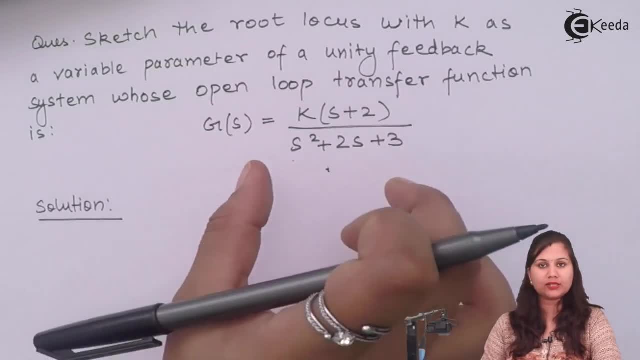 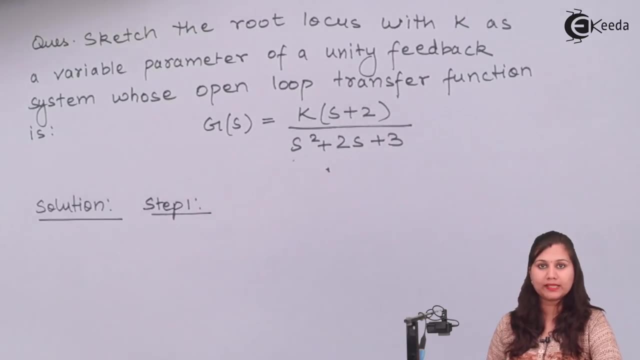 of the root locus. So let's try to find out the poles and zeros of this system and using this open loop transfer function. So our step number one is to find the poles and zeros. Now, zero is. we have to equate this numerator part to zero, so that s plus 2 equals to zero. 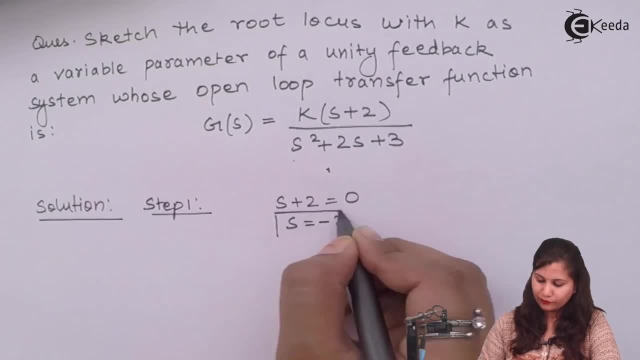 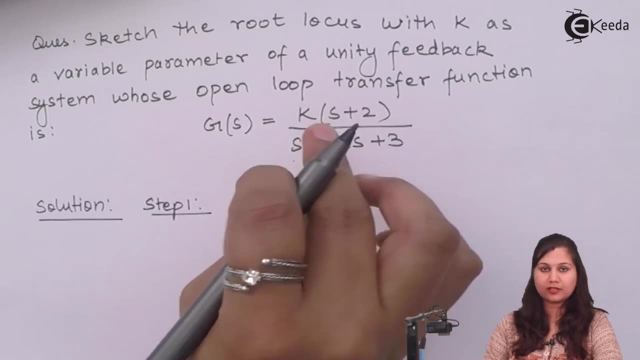 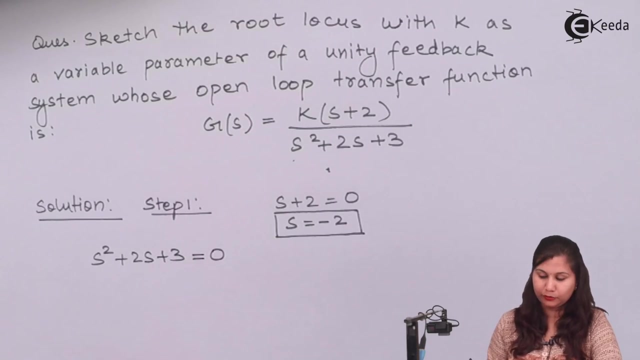 So we will have s equals to minus 2 as one of the zero of this system. Now for poles, we have to equate this denominator to zero. so we will have s square plus 2s plus 3 equals to zero. Now this is a quadratic equation, so we can have the roots of this. 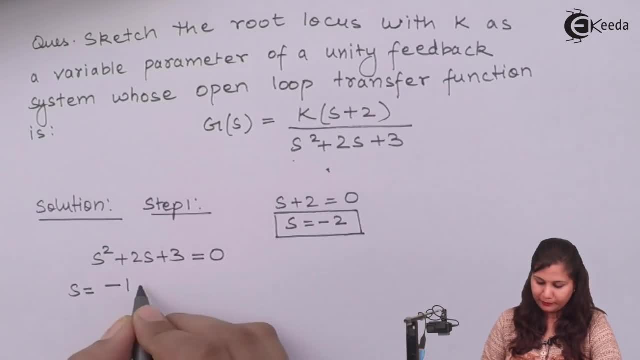 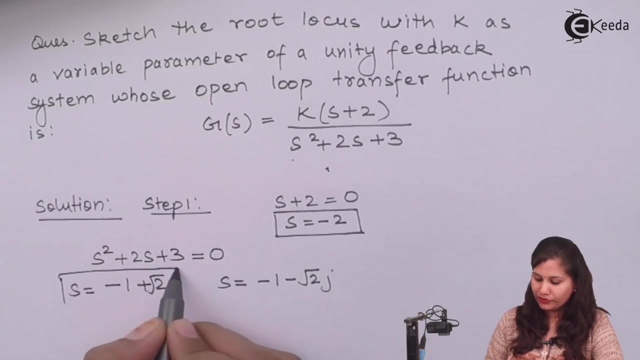 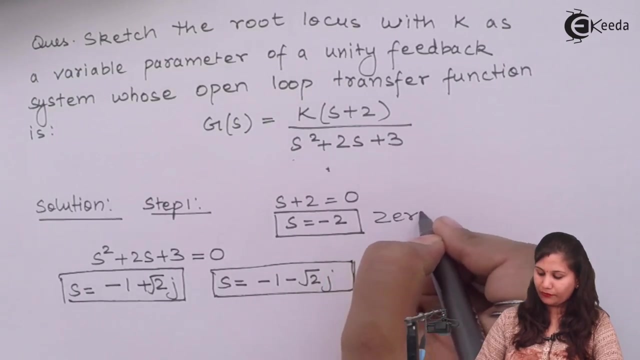 So if we calculate the roots, it will come out to be minus 1 plus 2j, and another root is minus 1 minus root 2j. Okay, so these are the two roots Of this equation, and the roots are called the poles. so we have two poles and one zero. 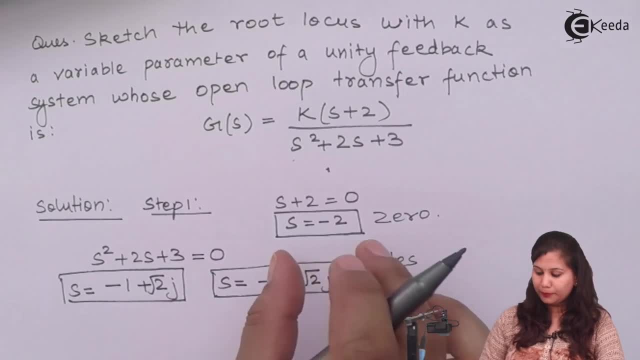 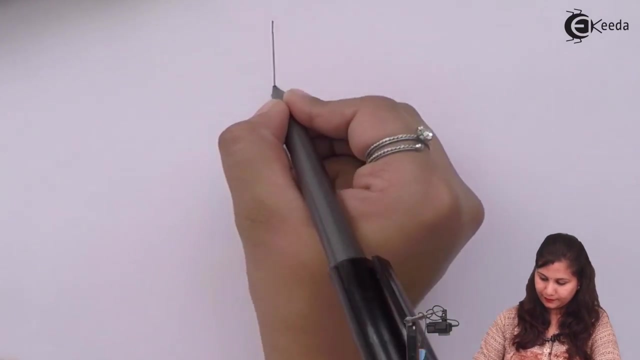 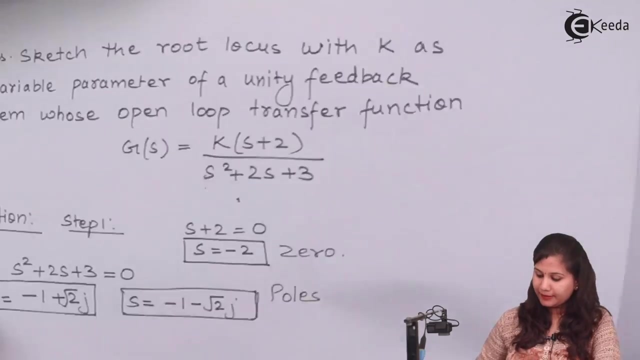 of this system. Now we are going to plot this zero and poles on the real and the imaginary axis so that we can get the location of these poles and zeros. Now, this is zero point. our zero is s equals to minus 2. so on, s equals to minus 2. this 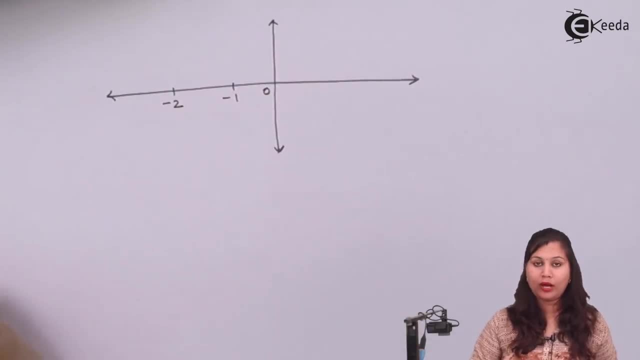 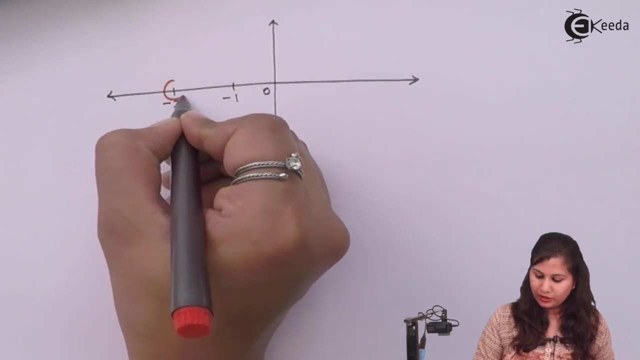 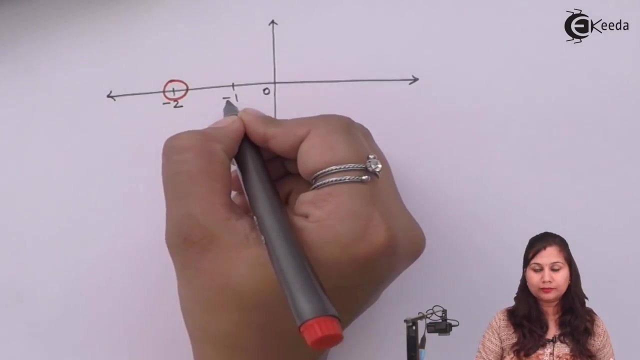 is minus 1, this is minus 2, so at s equals to minus 2. we are going to draw a circle because for zero we draw a circle here and the poles are denoted by the cross sign. So this is minus 1 and our pole is minus 1 plus 2j. 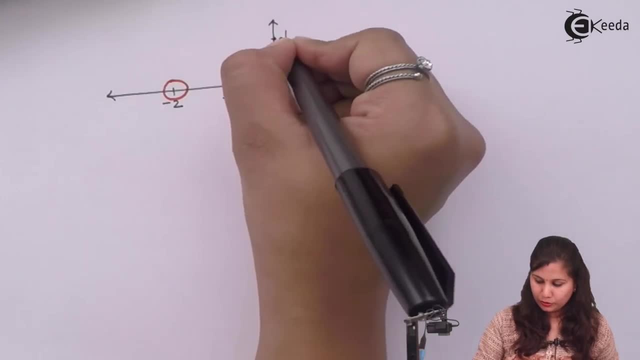 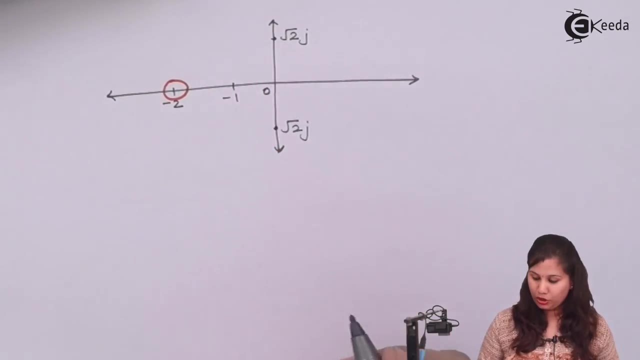 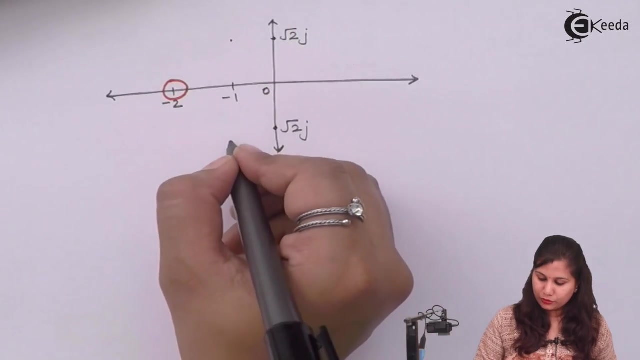 So this point is going to be root 2j and this is going to be minus root 2j, So minus 1 plus root 2j, so we will have this point and minus 1 minus root 2j, so we will have this point. 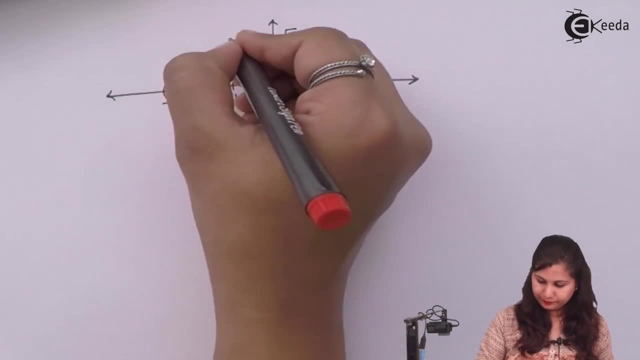 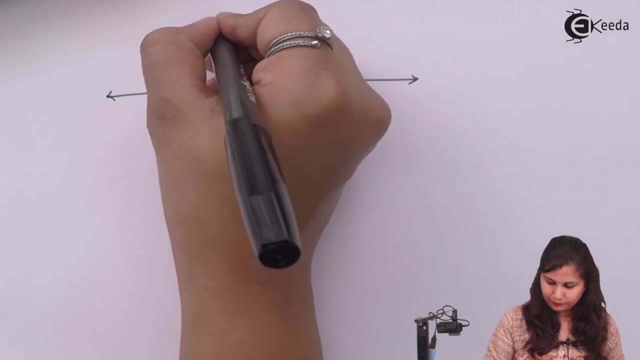 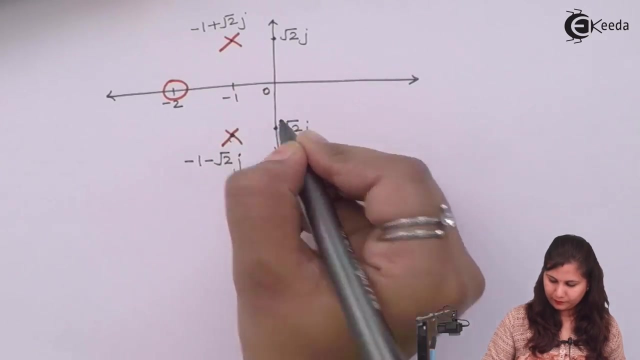 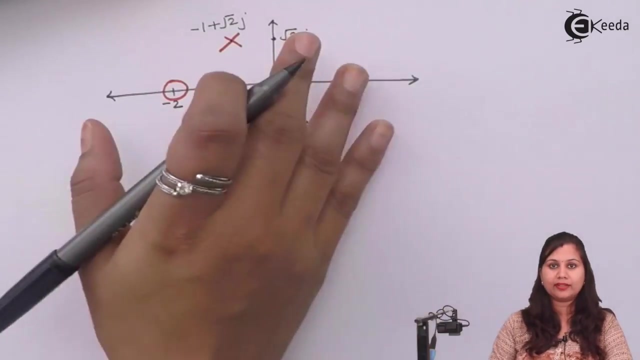 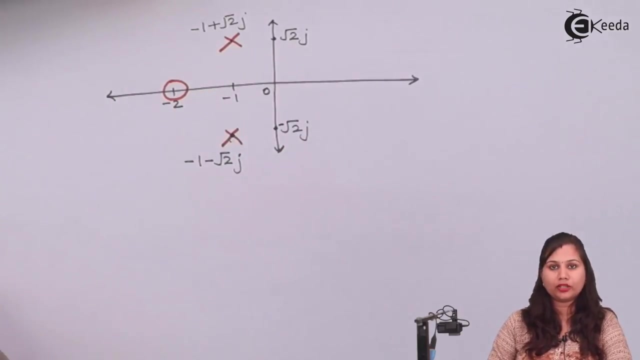 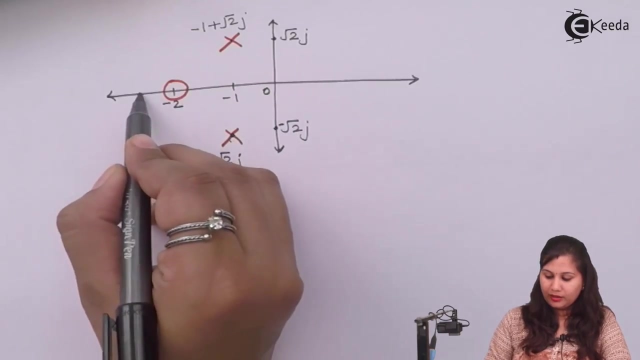 So these are our poles. Okay, so we have denoted the zeros and the poles on the imaginary and the real axis. okay, Now, for each of the poles and zeros, we are going to check the direction of the root locus By taking a point. so if we take a point here, then on the right hand side, the number of 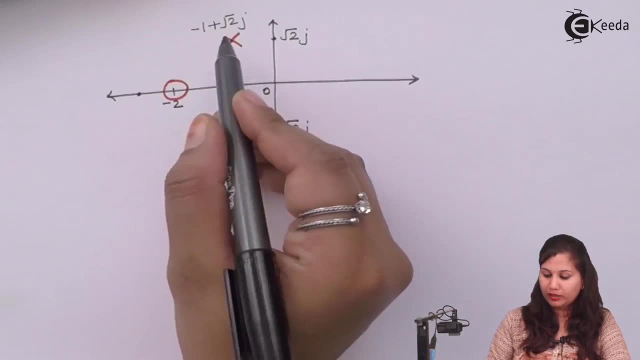 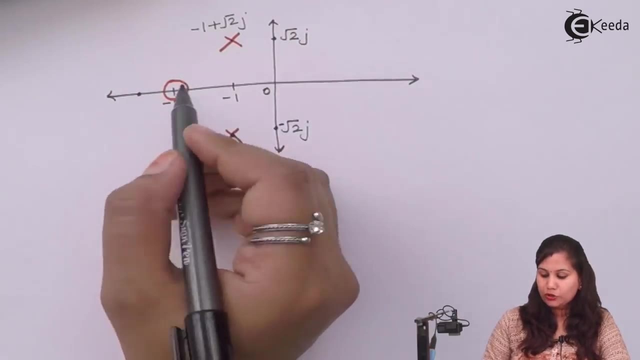 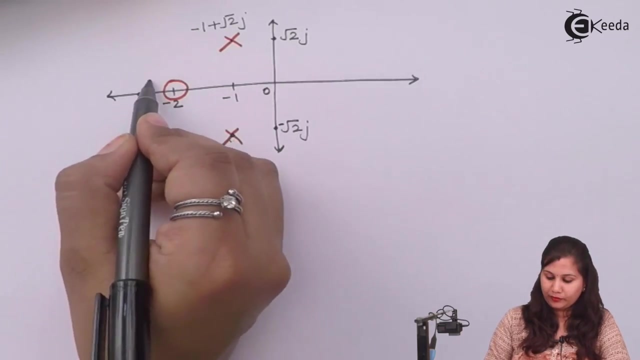 poles and zeros. if we calculate it will come out to be 1,, 2 and 3.. So 3 poles and zeros are located on the right hand side of this point. So the direction of the root locus for this zero, it will be in this side. this is for this. 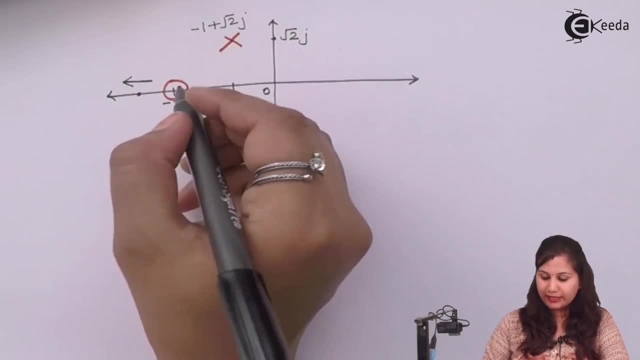 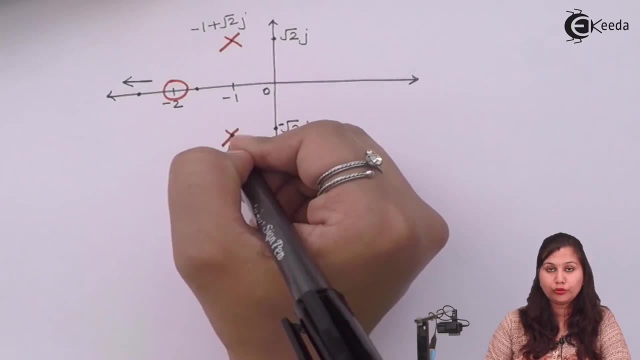 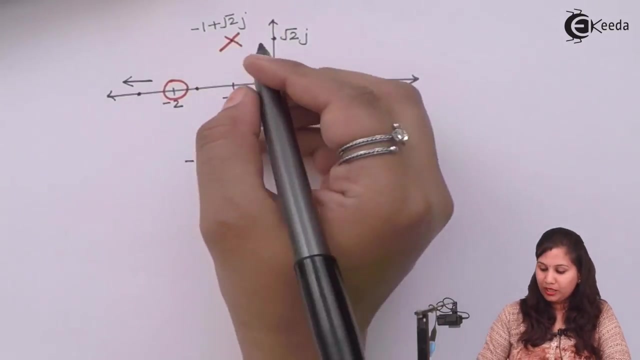 zero. Now, if we take a point on the right hand side of this zero here, then the number of poles and zeros on the right hand side of this point are 2.. So the direction of root locus will be for this side, for this zero. 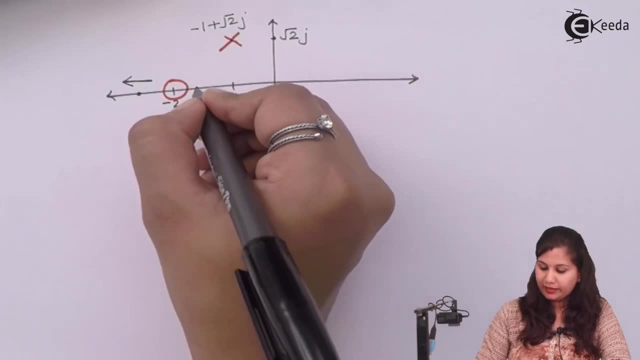 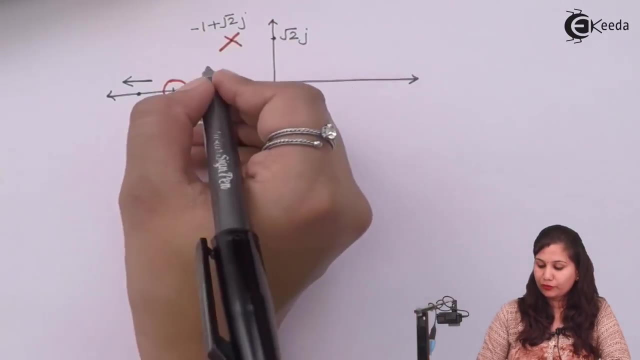 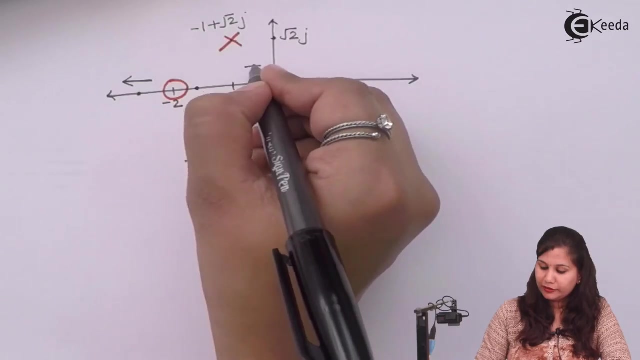 Now, if we check for these two poles, then again, taking this point, So on the right hand side we have the two poles, so the direction of root locus will be this side, Because it is the number is even. so, the direction of root locus will be this side for these two. 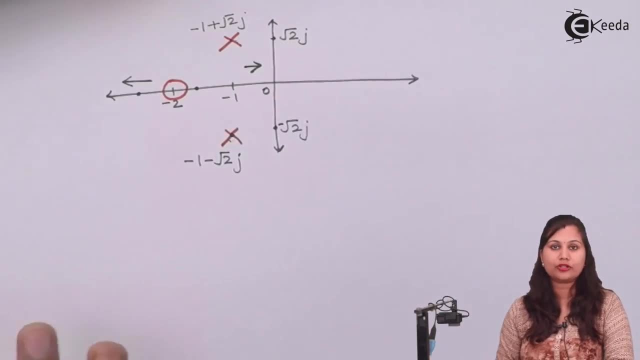 poles. So in this way we are checking the direction of the root locus. Now our step number 2, that how many branches of root locus will be there. Now, if we see we have the two poles, So the number of branches of root locus. 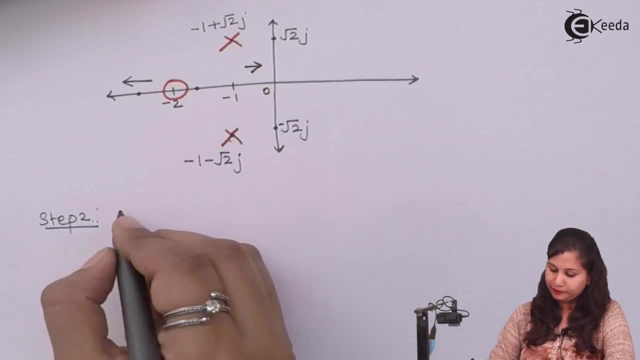 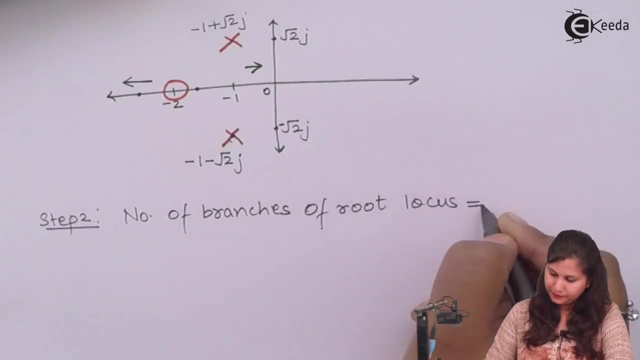 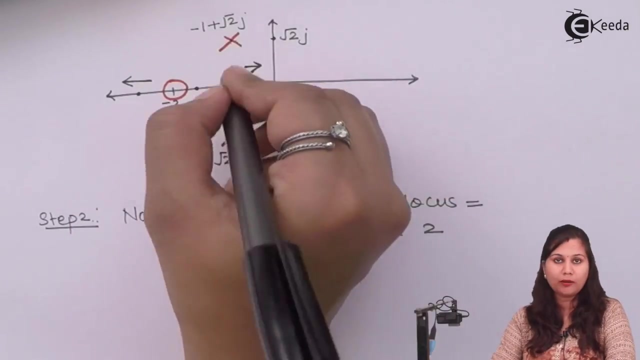 So the number of branches of root locus is equal to the number of poles, And number of poles for this system are 2.. So there will be two branches of root locus, Now for both these poles, because their location is almost same in 90 degrees to each other. 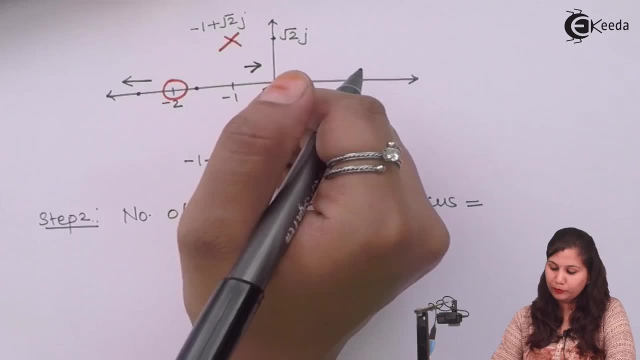 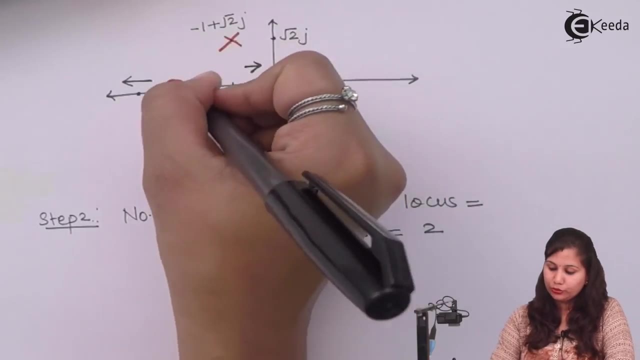 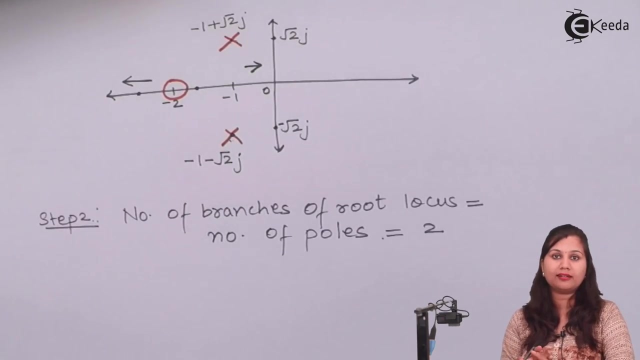 So if we take the root locus For these two poles, then they are going to meet at some point, or, and then we are going to calculate the breakaway point, that is, the point where the two branches, they are intersecting with each other. okay, So our step number 3 is to calculate the breakaway point. 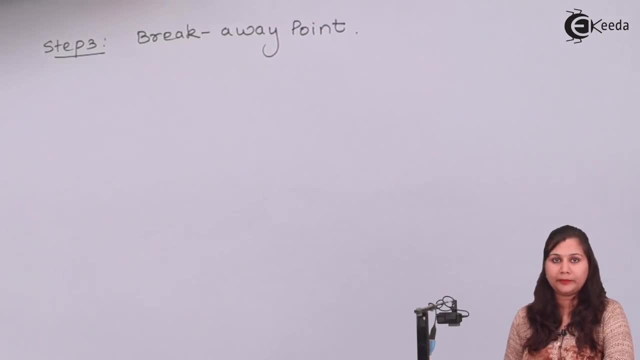 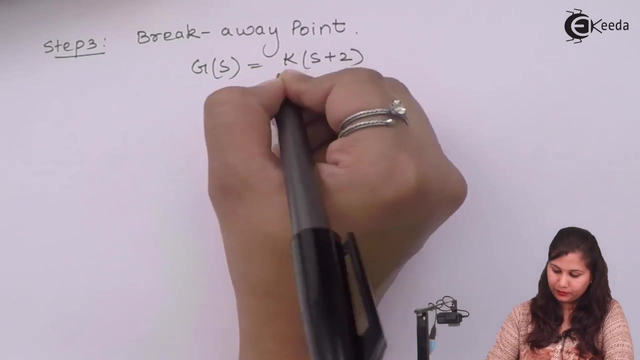 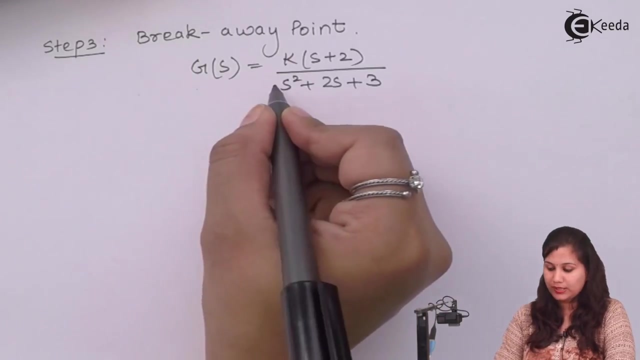 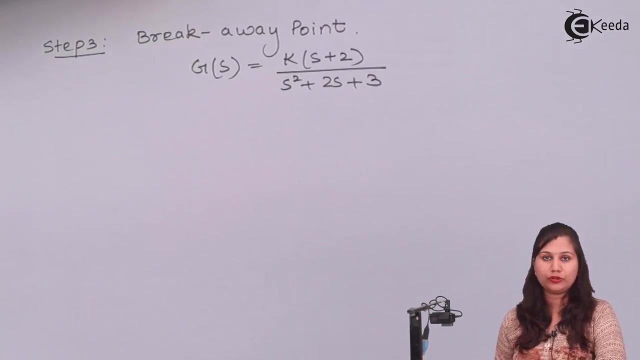 Now to calculate the breakaway point, we will use the transfer function given to us. We are going to differentiate this transfer function with respect to S, and then we are going to equate that that differentiation equals to 0.. So just differentiate this G with respect to S. 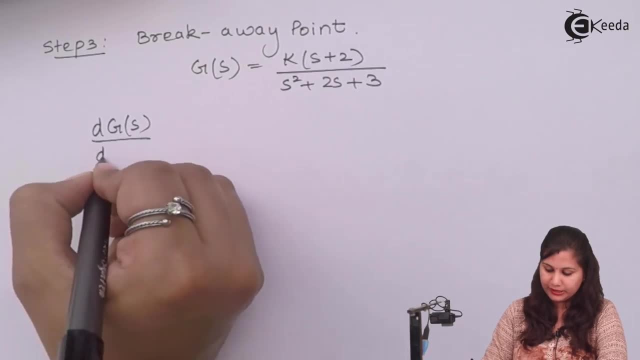 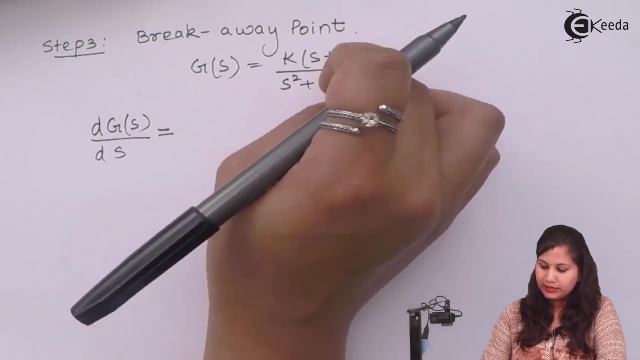 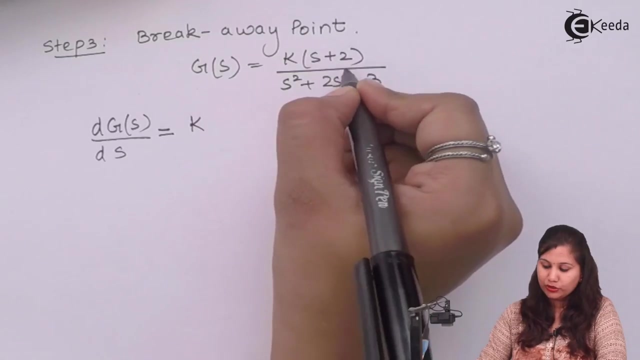 Okay, So it will be DGS upon DS, So its differentiation will be first K into this S plus 2 differentiation, and then denominator will be as it is. So K, S plus 2 differentiation will be S, it will be 1 and 2 it will be 0.. 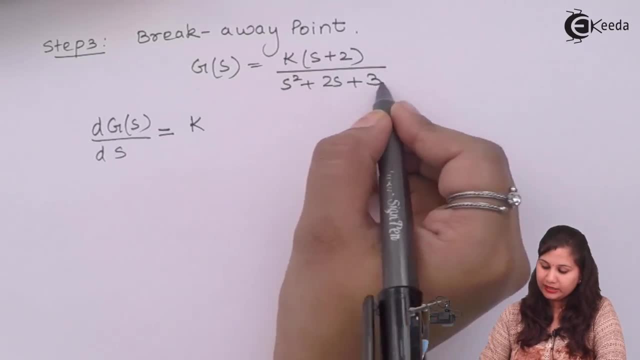 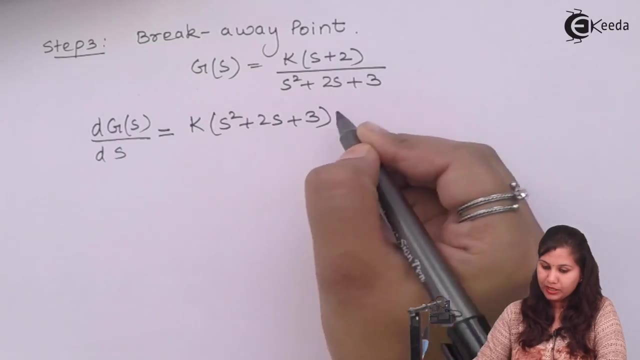 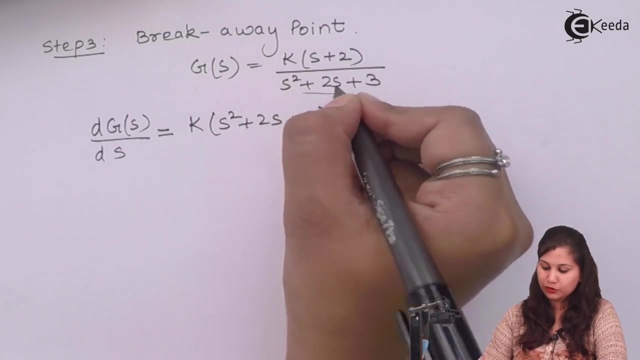 So we will have only 1 there and then it's. the denominator part will be as it is, So S is equal to 0. So it will be 1 S square plus 2 S plus 3.. Then we will have minus sign and then differentiation of this denominator term will be 2 S plus. 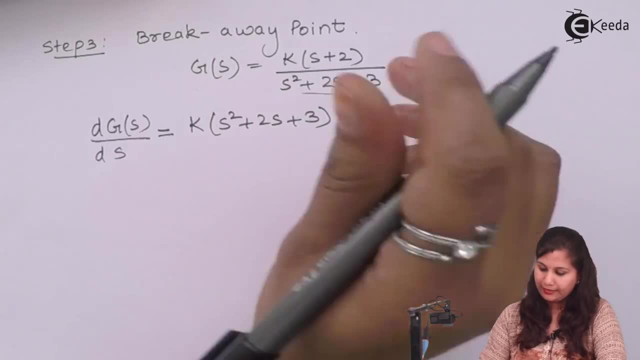 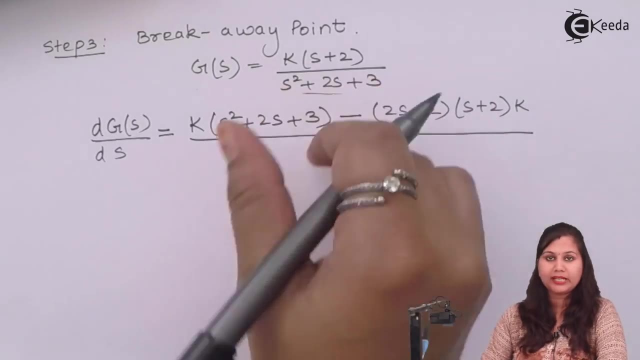 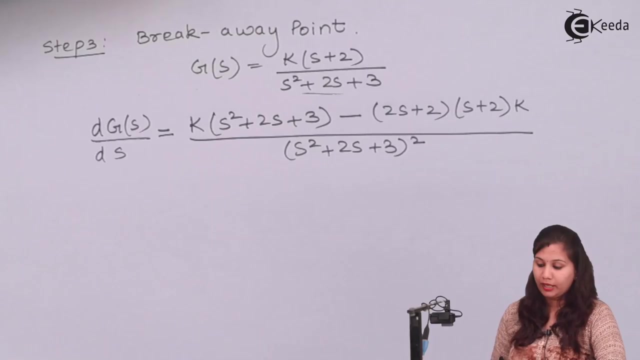 2. And this numerator part will be as it is Upon denominator square. Now we are going to equate this denominator term, So This denominator term will be. This numerator term will be. This denominator term will be. This denominator term will be. 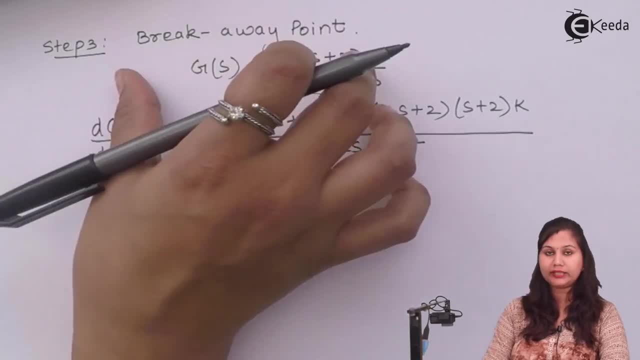 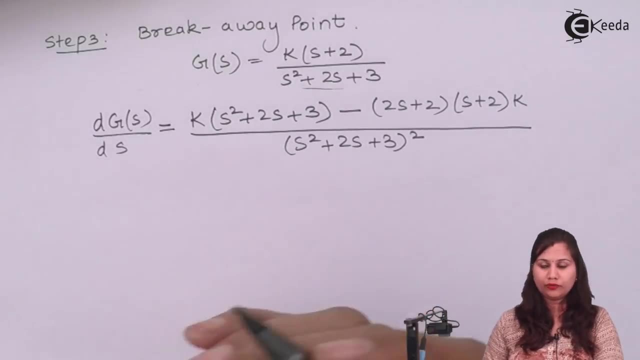 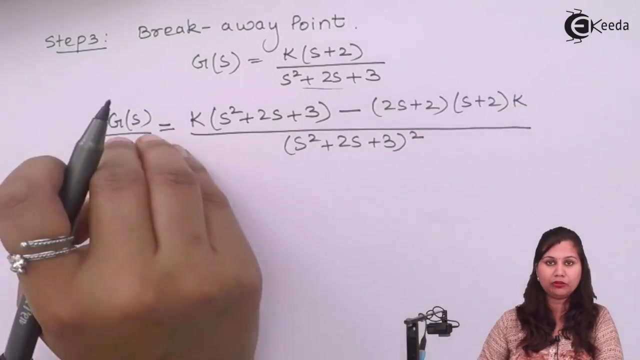 DGS upon DS equals to 0 to calculate the breakaway point. so putting this whole equation equals to 0. so equating this to 0 we will get the denominator will become 0 and if we take common from these two terms then K will be common. so 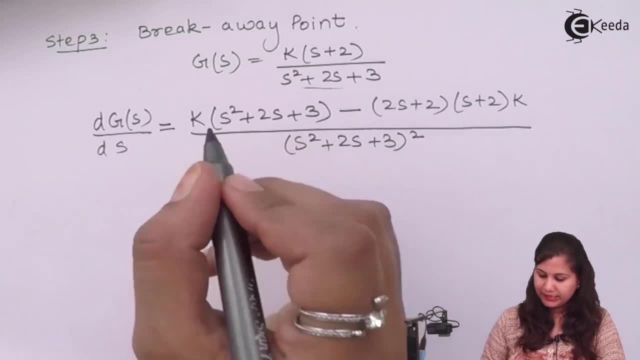 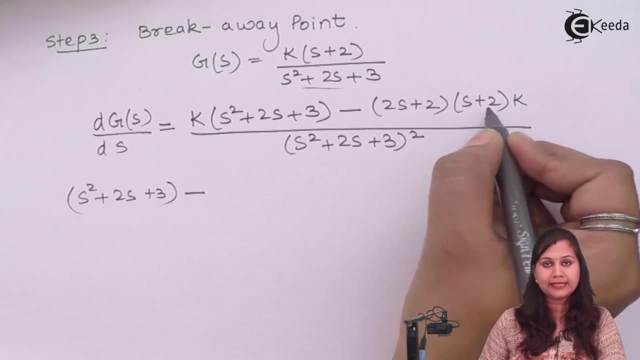 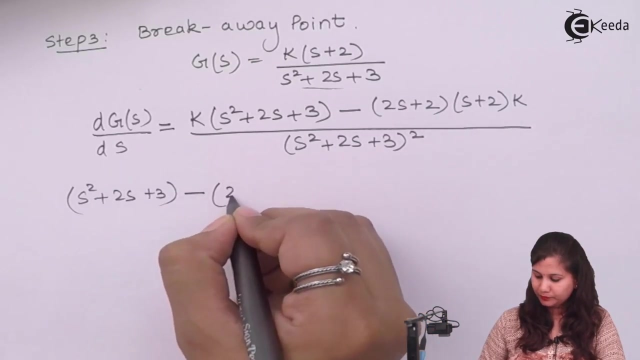 it will also be equal to 0. so we are left with s square plus 2s plus 3 minus multiplied these two, so we will have 2s square plus 4s plus 2. this is 4S. this is 2s. so 4S plus 2S is 6S plus 2 to 4, so we will have this. 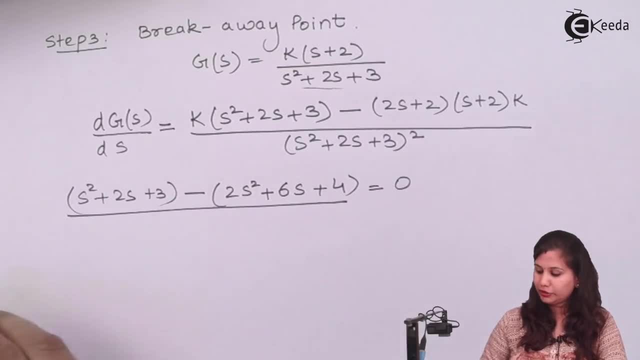 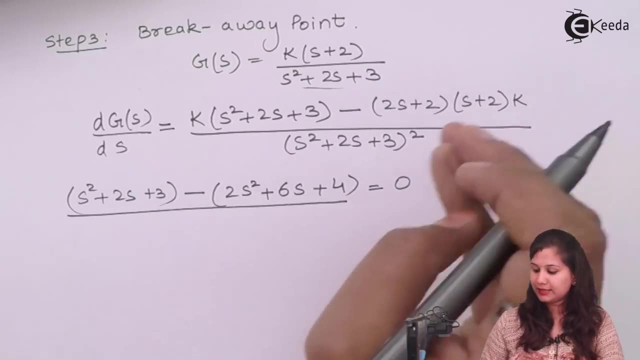 equals to 0 the denominator part, because we have on the right hand side we have zero. so we will get the denominator part because we have on the right hand side we have zero. so we, when we cross, multiply this, this denominator term is going to become 0 and k is also cancelled out. 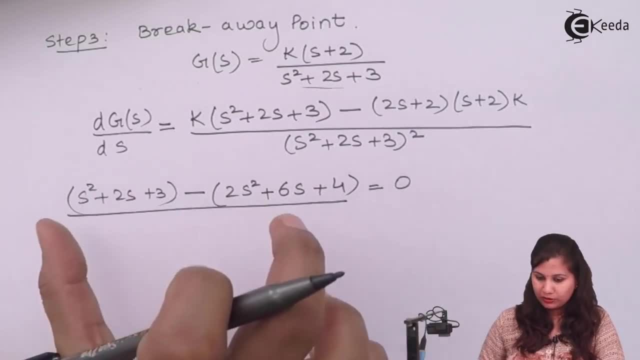 because we can take it as common. So when we solve this we are going to get this is s square minus 2s square, so it will be minus s square, 2s minus 6s, so minus 4s, and 3 minus 4s minus 1 equals. 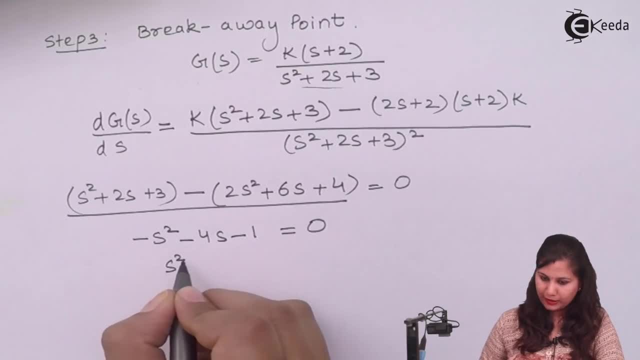 to 0. or we can say: this is s square plus 4s plus 1 equals to 0.. Now we can solve this quadratic equation to get the value of s. so s will be equals to minus 3.73.. So this is the breakaway point. 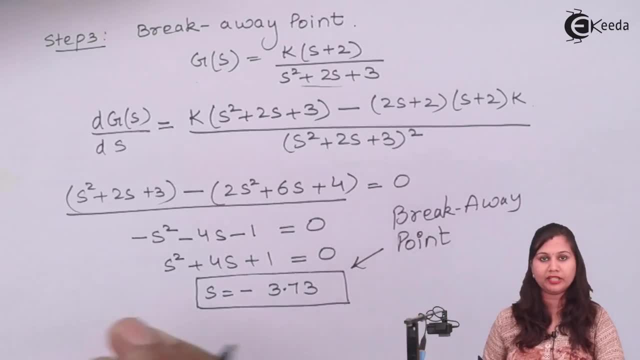 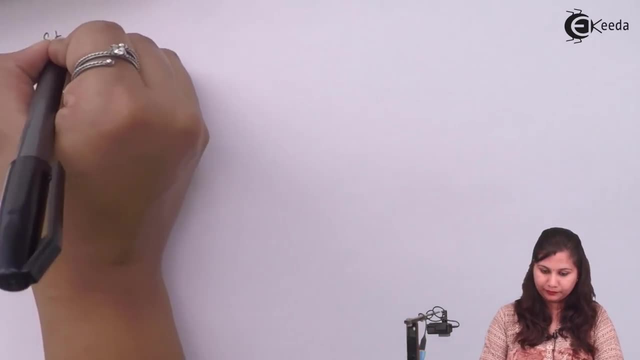 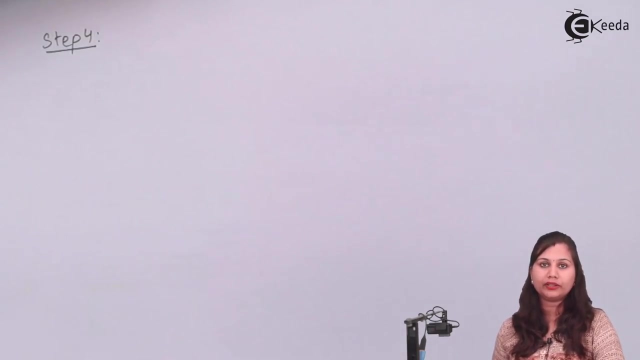 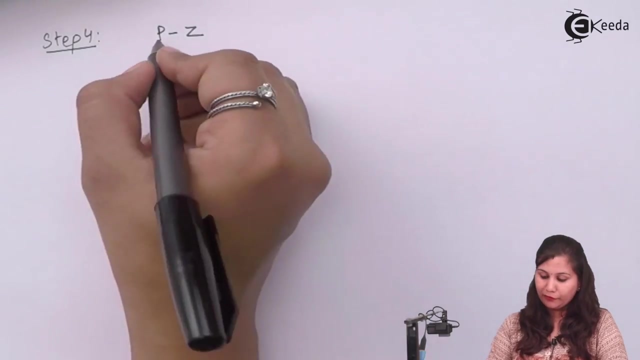 So we are going to use this value when we will draw the root locus. Now our step number 4.. Step number 4 is to determine the asymptotes on the real axis. So how many asymptotes are there? We will calculate p minus z. Now number of poles is 2 and number of zeros is 1.. So 2 minus 1 it. 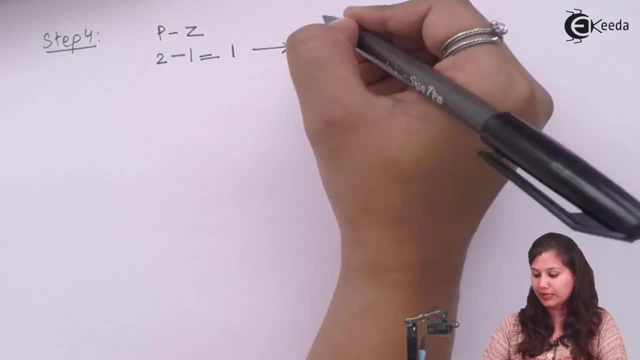 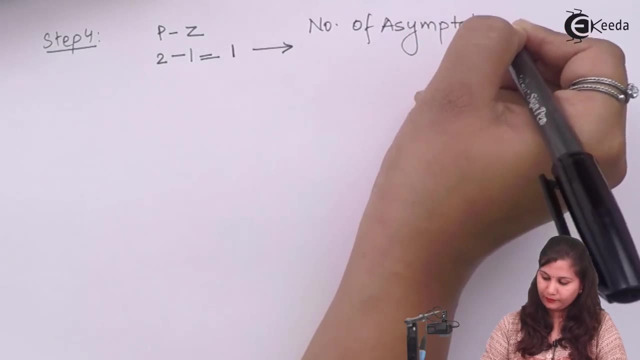 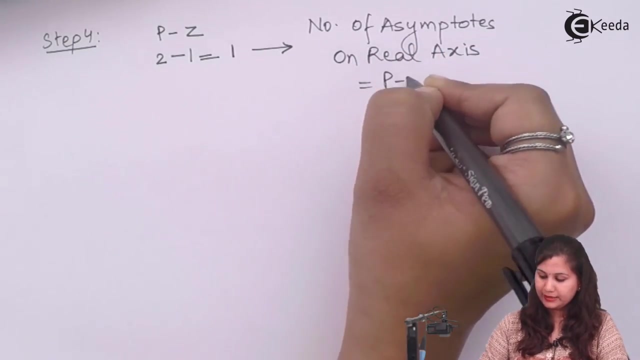 is equal to 0. So we are going to use this value when we draw the root locus. Now our step number 4 is to determine the asymptotes on the real axis. So the number of asymptotes on real axis. it is equal to p minus z, that is number of poles minus number of zero. and we have 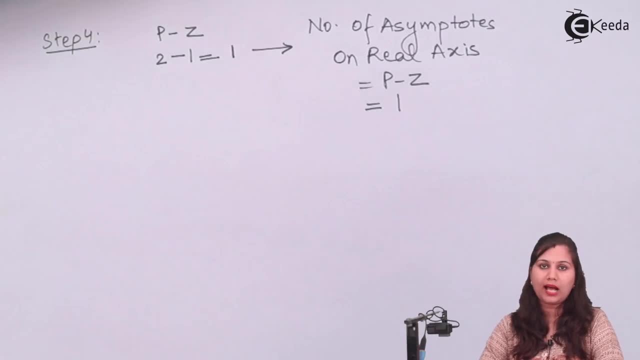 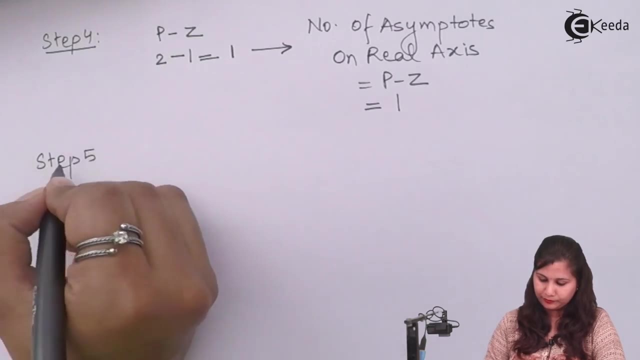 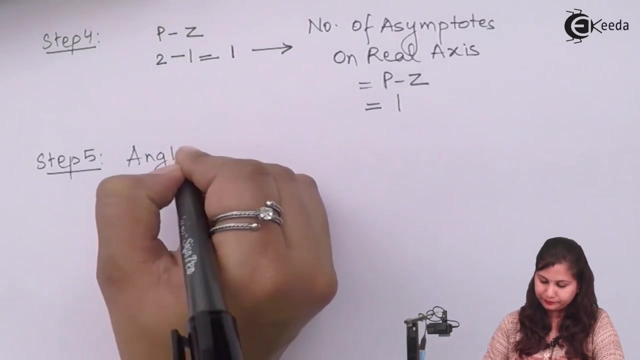 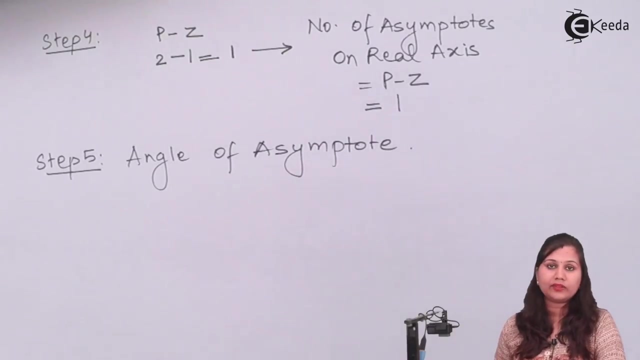 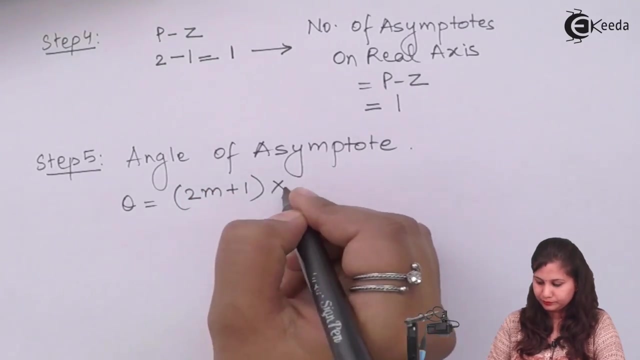 calculated it is 1.. So there is only one asymptote for this system. Now next step is step number 5. We have to calculate the angle of asymptotes. For this we have the formula theta equals to, theta equals to. Now here: this n is equal to theta, So this n is equal to theta. So this n is equal to theta. So this: 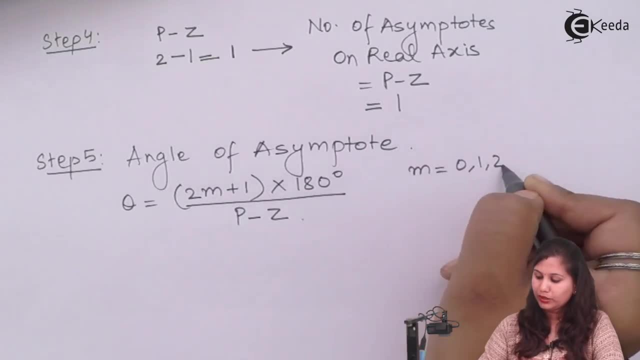 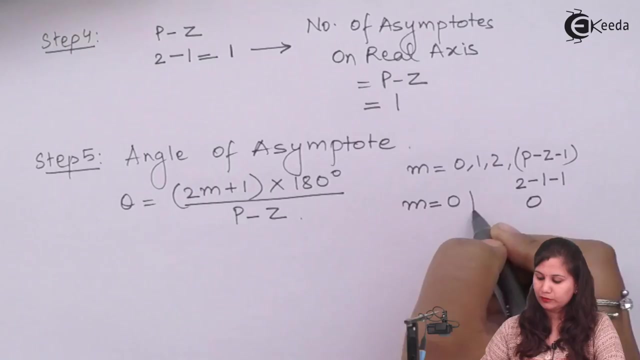 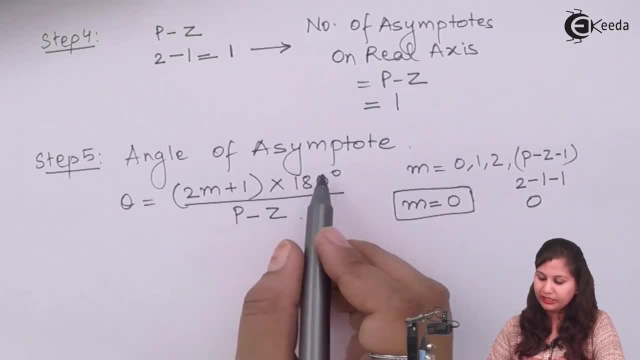 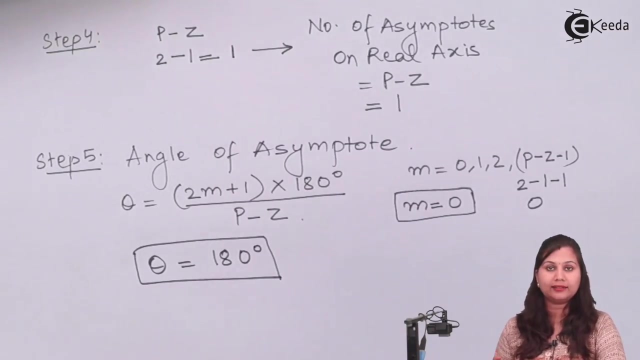 M equals to zero, So it will be 1 into 180 degree upon p minus z is. we have already calculated, it is one. So this theta angle, it is coming out to be 180 degrees. So the angle of asymptote, that is the angle the asymptote is making with the real axis, it is 180 degrees. So this real axis is the asymptote for this control system, For the system. 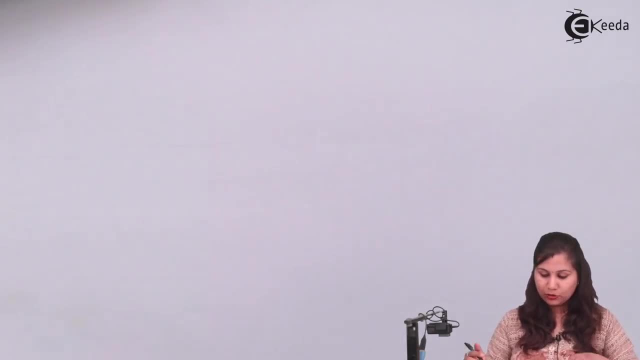 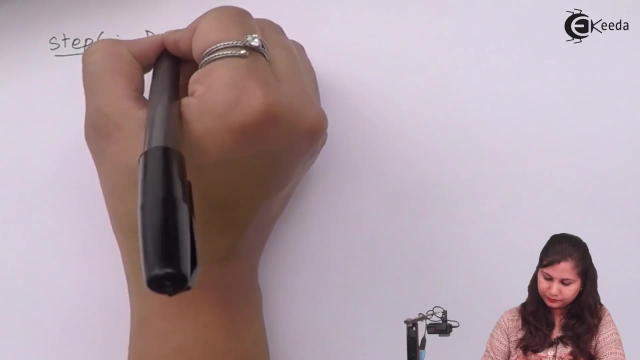 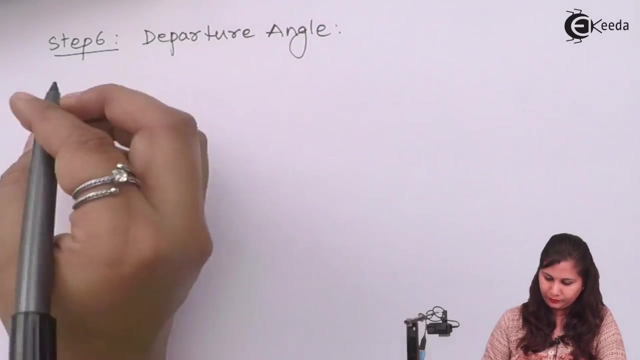 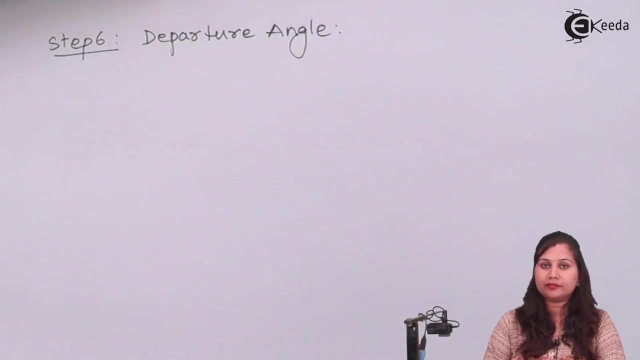 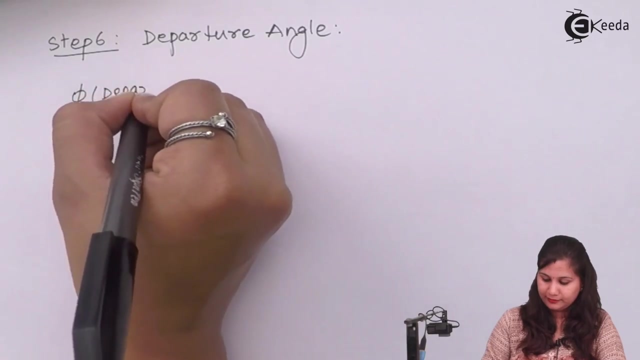 which is given to us Now. next step is to calculate the angle of departure, Because this system is involving two complex poles, so we will have to calculate the departure angle for the two complex poles. so first we will have the phi departure angle. This angle 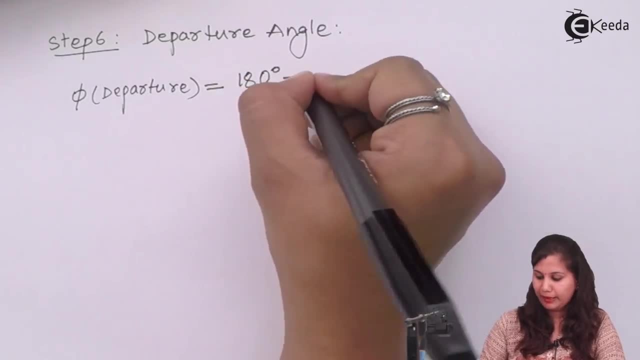 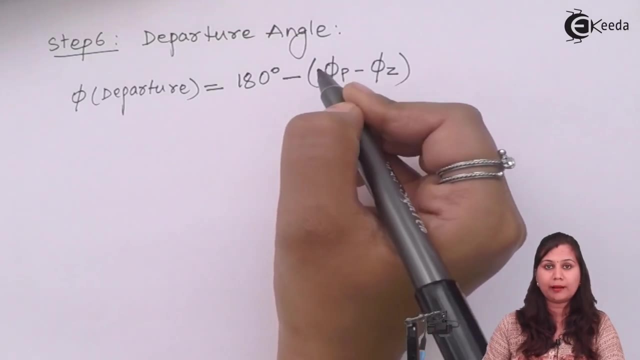 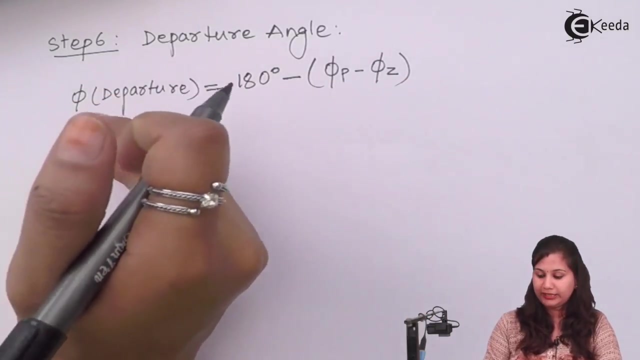 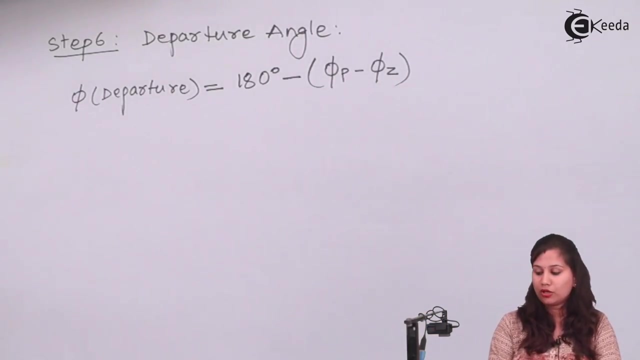 is calculated by using the formula 180 degree minus phi p, minus phi z, where phi p it is the sum of the angles subtended by the rest of the poles- for the pole which we have calculating, the departure angle, and phi z is the sum of the angles subtended by all the zeros on. 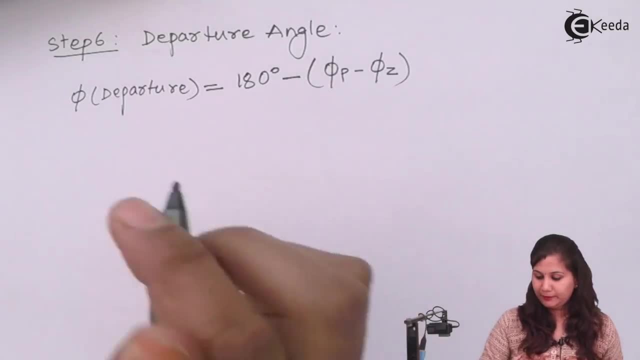 this complex pole. So if we take phi p for the complex pole, it will come out to be 90 degrees and phi z 1 is coming out to be 55 degrees, How We can see here when we have located the poles and zeros. 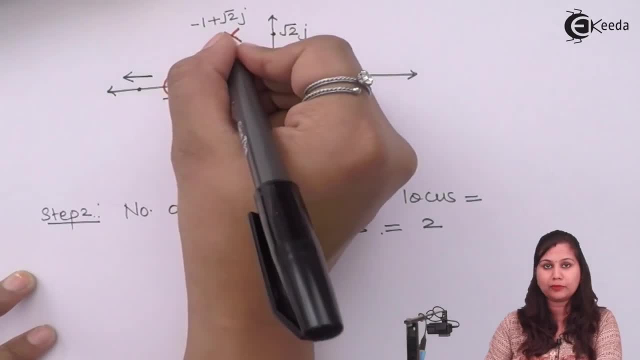 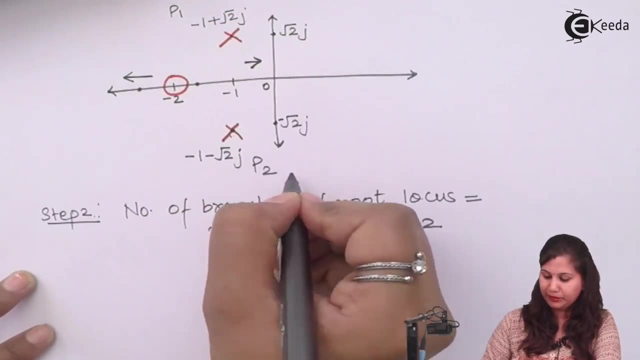 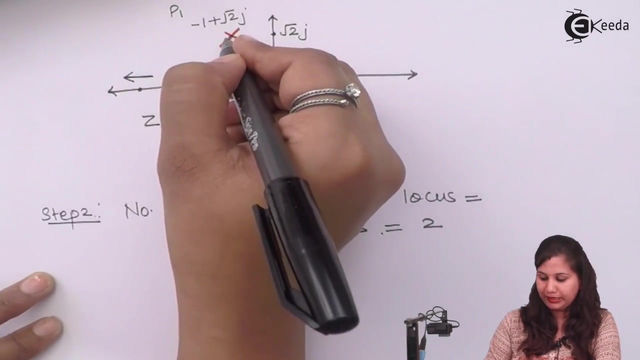 the real and the imaginary axis. so for this complex pole we are calculating the Phi P1. suppose this is our first pole, P1, this is pole second P2, and this is the zero Z1. so Phi P1, it is the angle subtended by. this is Phi Z1 and this is 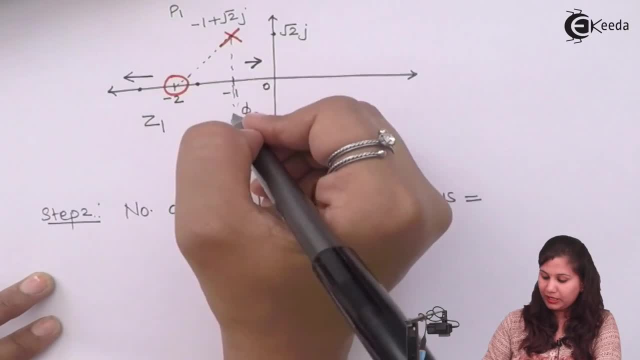 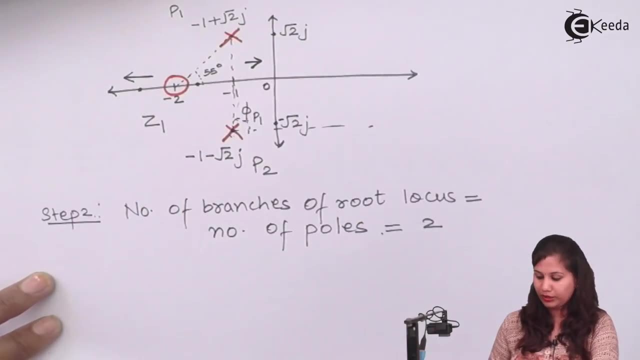 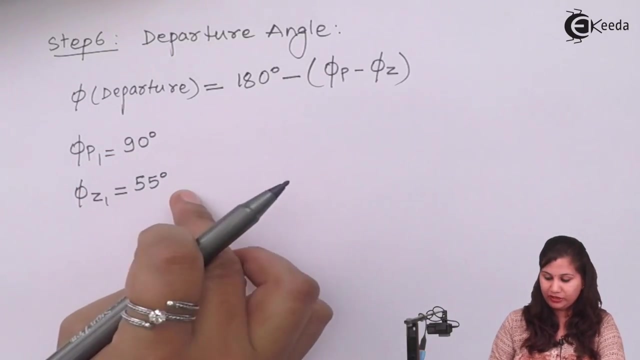 Phi P1. so this is coming out to be 90 degrees, and if we calculate this angle, then it will come out to be 55 degrees. okay, so here we have written Phi P1 as 90 degrees and Phi Z1 as 55 degrees. so let's put the value of these angles here. 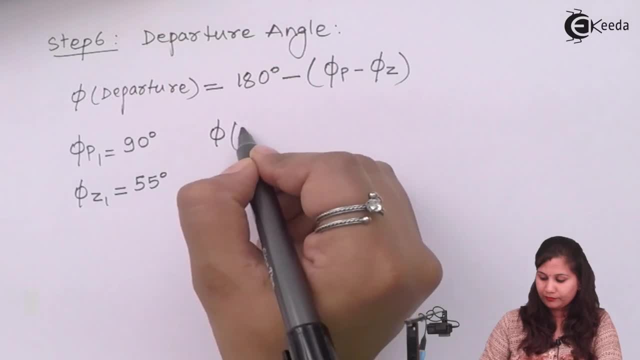 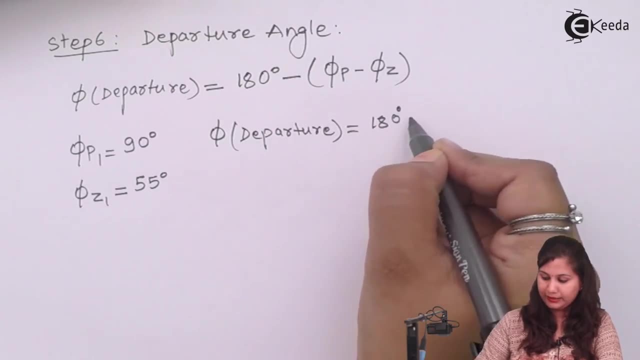 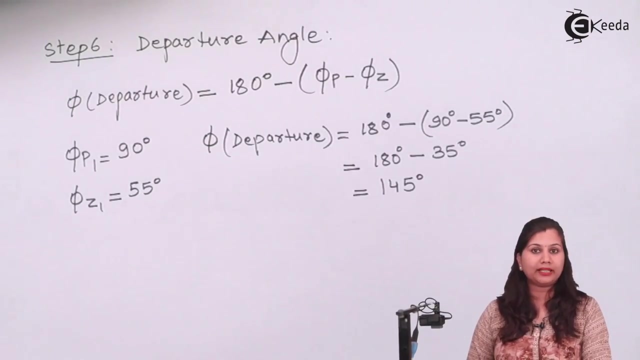 so here we will have 180 degrees: 180 degrees minus 90 degrees, minus 55 degrees, so this will be 90 minus 55 will be 35 degrees. so Phi departure is 145 degrees. so we have calculated all the variables like departure angle, breakaway point, angle of asymptotes. so using all these, 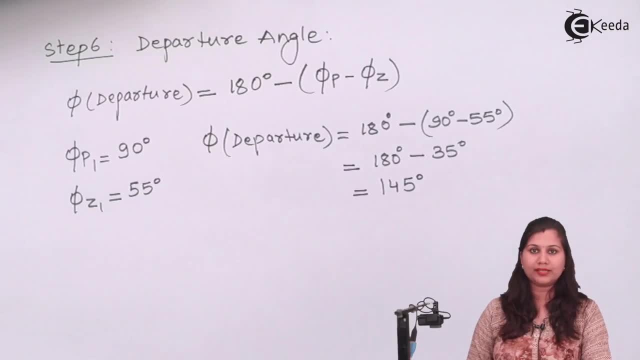 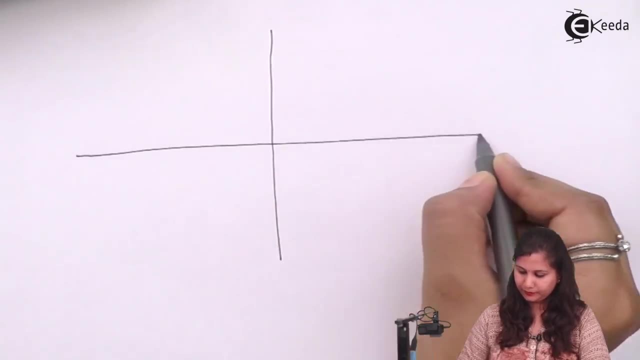 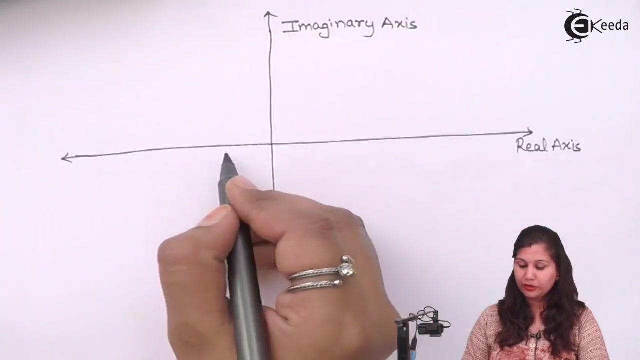 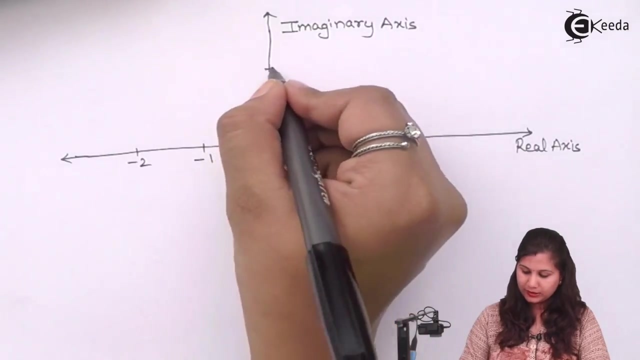 variables. now we are going to draw the root locus of the system. this is our imaginary axis and this is the real axis. so now we are going to plot our poles and zeros here. so this was minus 2, this is minus 1, this is root 2j and this is. 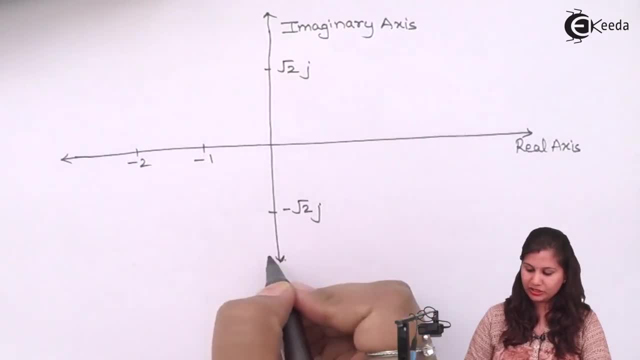 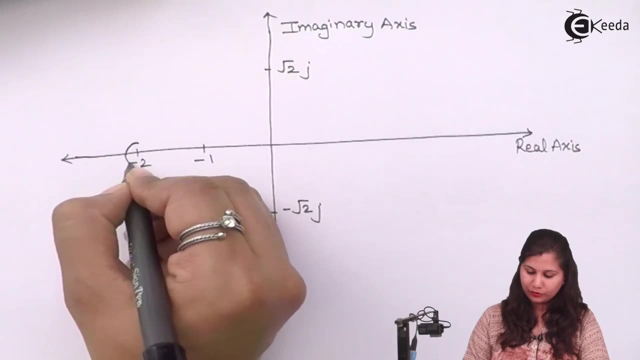 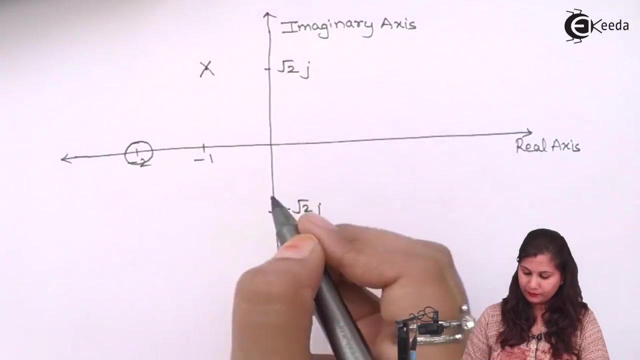 minus root 2j. so this is imaginary axis, this is real axis. we have marked the points. so s minus 2 was our zero, and on minus 1 plus 2j we have the pole, and minus 1 minus root 2 j we have our second pole. okay, we are going to write. 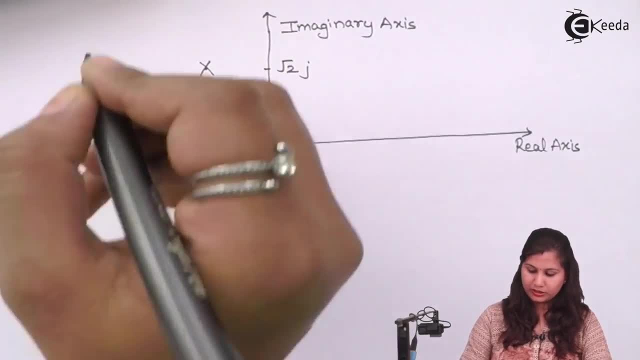 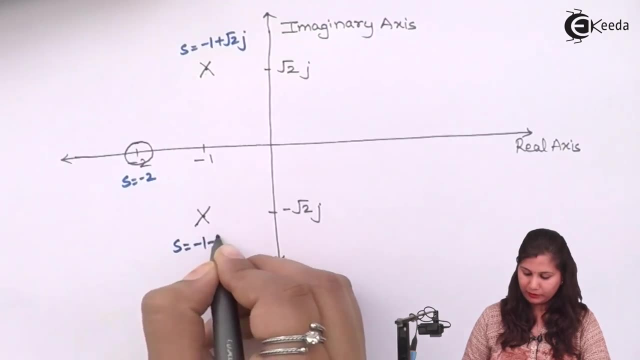 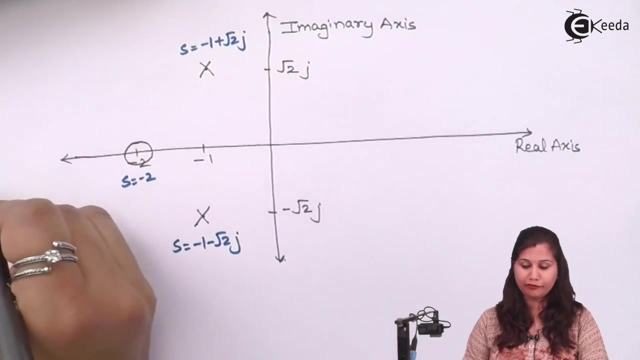 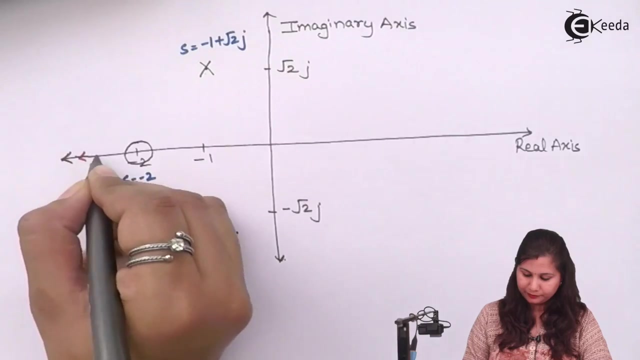 it here: s equals to minus 2, s equals to minus 1 plus root 2j, and s equals to minus 1 minus root 2j. Now for this 0,. the direction of the root locus is towards the infinity. So here we are going to mark the points, mark its direction here. 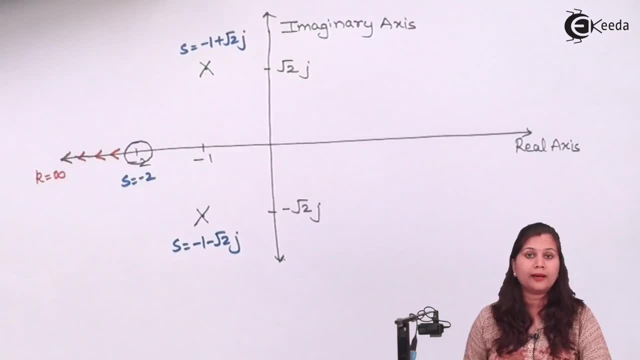 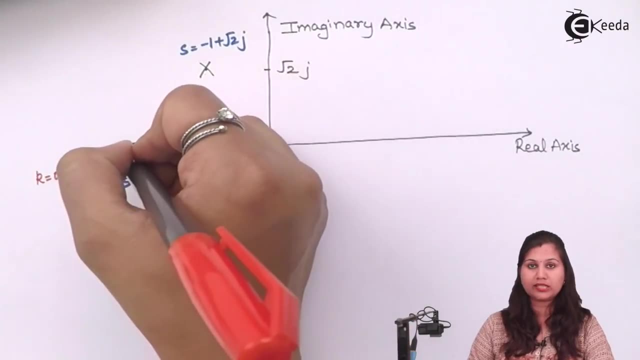 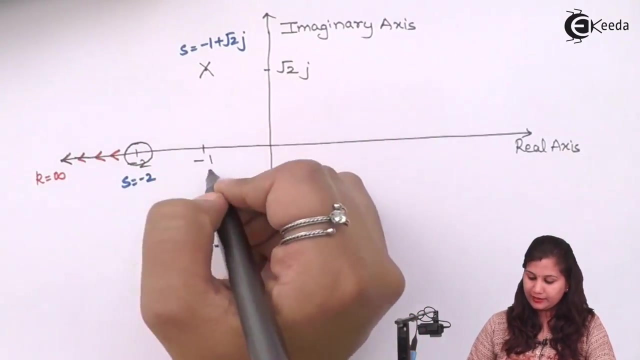 This is k equals to infinity, Because the root locus it always starts from the pole and terminates at either infinity or towards the 0. So here this root locus will be for this pole and this pole it is towards this 0 point. 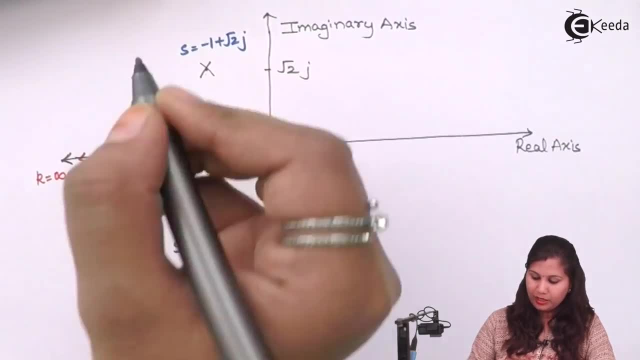 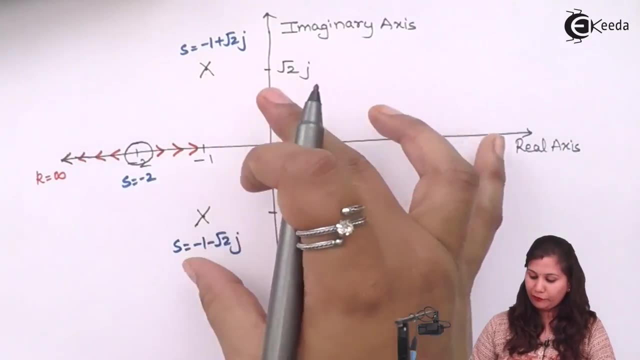 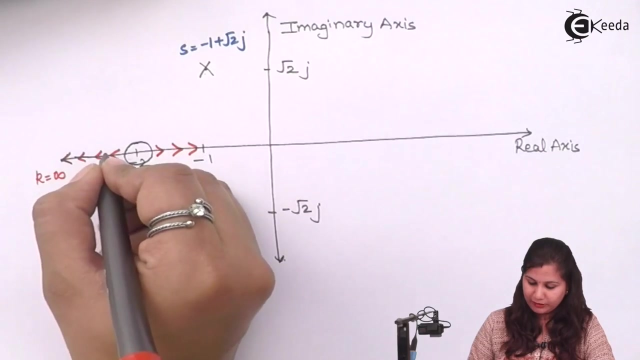 So here we have this Now for this pole. it will come towards this side and this side because our breakaway point for these two root locus branches it is at minus 3.73.. So minus 3.73 point will be: this is minus 2, so it will be somewhat here. 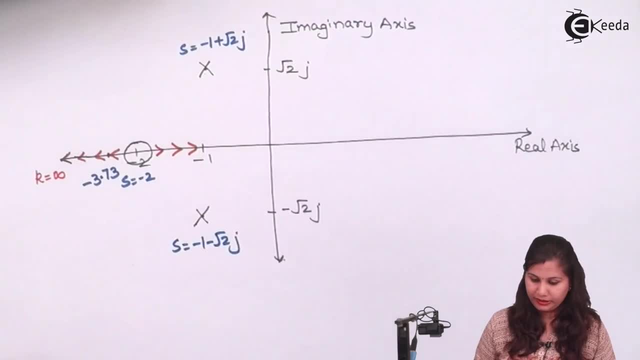 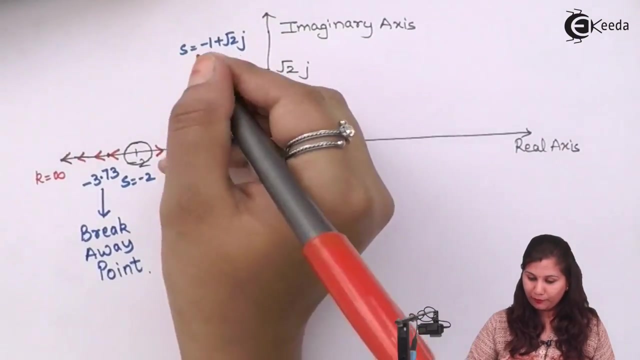 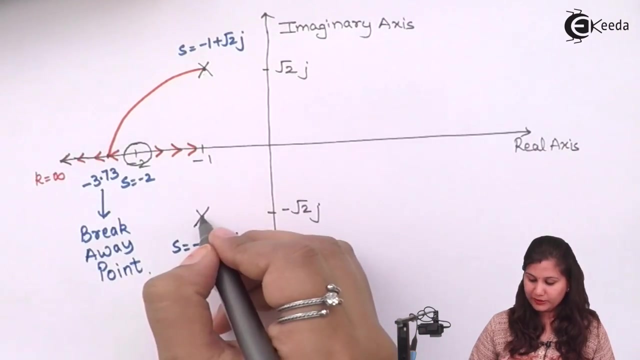 This is minus 3.73, which is our breakaway point. Now the root locus. Now the root locus. from this pole, it will come at this breakaway point and also, starting from this pole, it is also going to come towards this breakaway point. 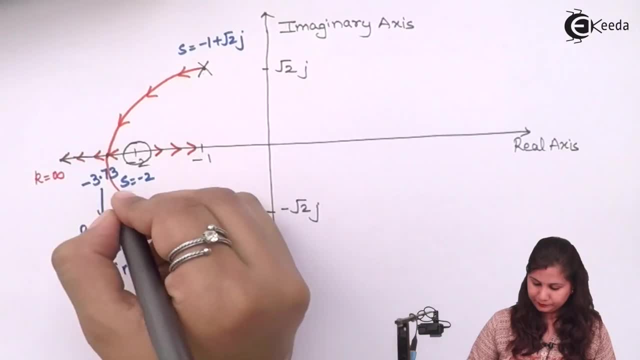 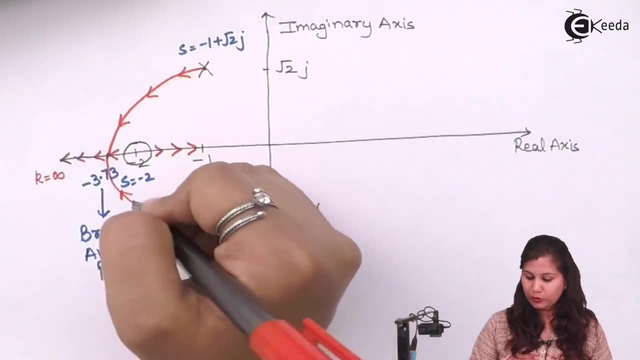 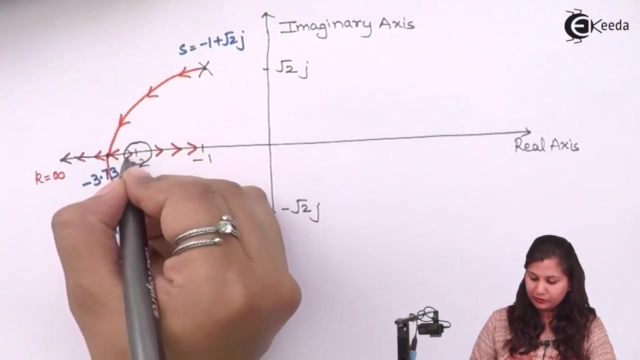 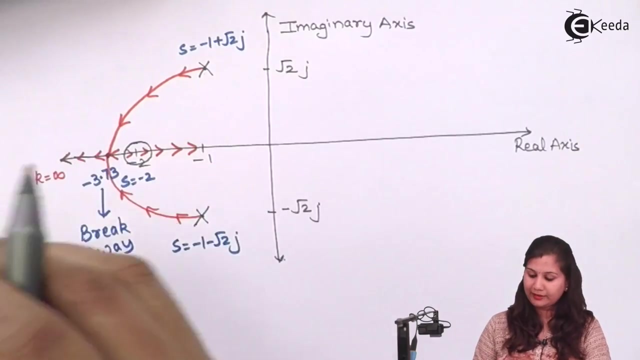 Its direction will be like this. and its direction will be like this. Now, coming from all, from these two poles, the root locus branch, it will go towards this 0 point. So we have Drawn the direction here. So, all these two root locus branches, they are going to meet at this breakaway point. 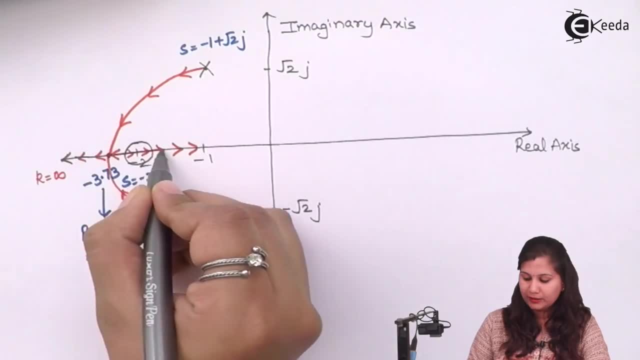 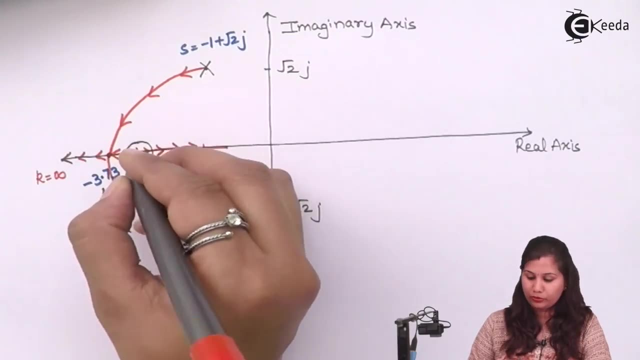 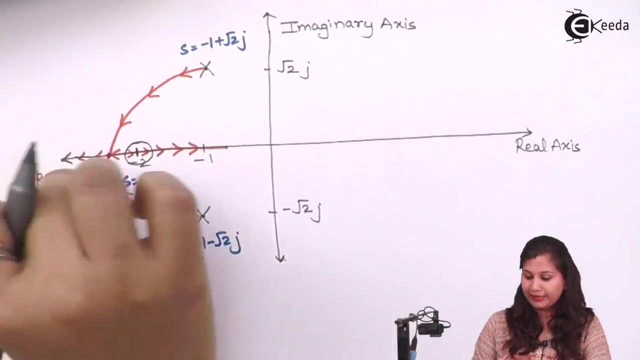 and then they are going to come towards this line, Okay, And then it's going to end up at this minus 2.. Okay, So this is the root locus of this system. Now, our asymptote was the minus 180 degree. 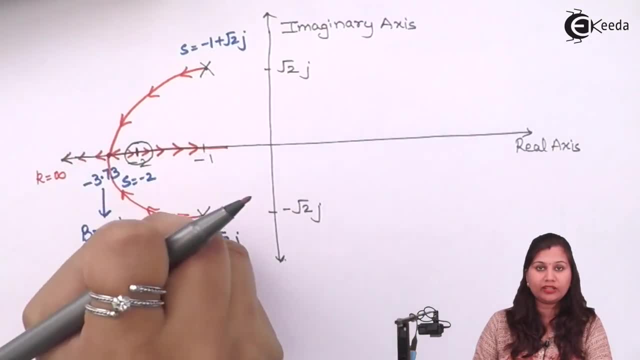 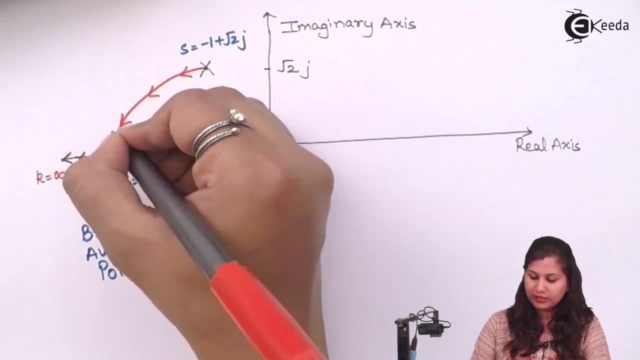 That is the angle which The asymptote is making with. the real axis is minus 180 degree. So this will be the asymptote here and starting from the pole, the asymptote is going to terminate at this point as equals to minus 2 the 0..